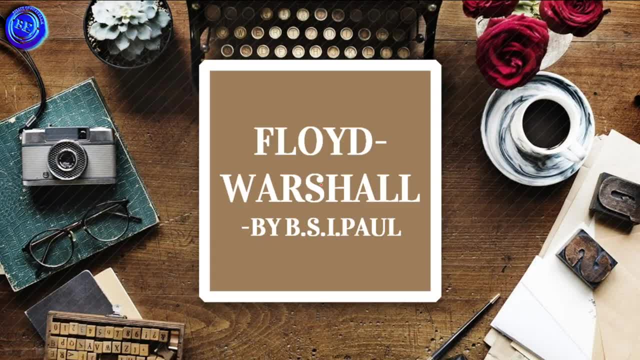 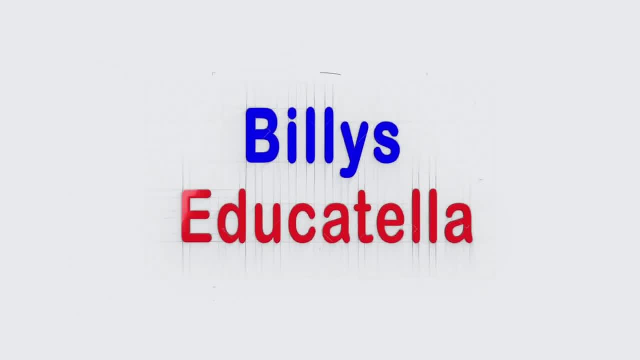 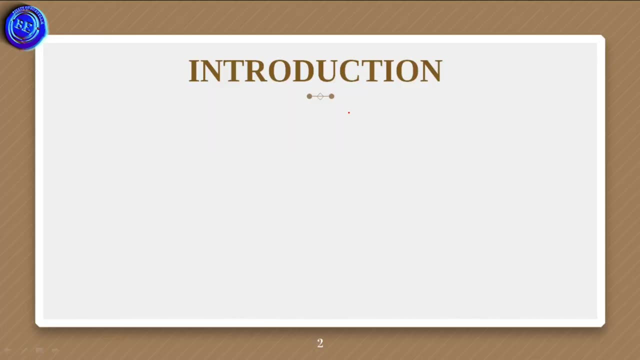 Now let us discuss the topic of Floyd Verschel Algorithm. Intro, Coming to the introduction part of Floyd Verschel Algorithm. What is a Floyd Verschel Algorithm? So it is an algorithm for finding the shortest path between all pairs of vertices in a weighted 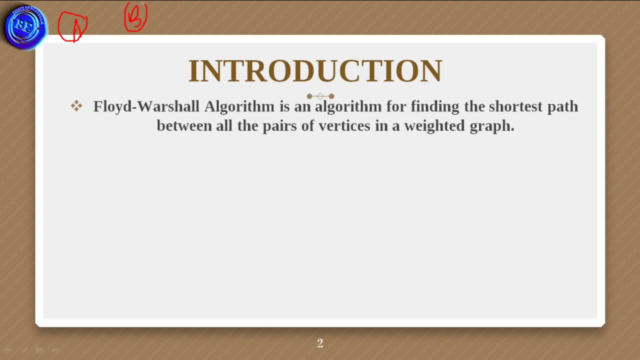 graph. Here I am considering a graph named as A, B, C and D, And we have some edges between the vertices, So this algorithm will find the shortest path for all pairs of vertices. That means from A to B, A to C and A to D. So here the shortest path from A to B is calculated. 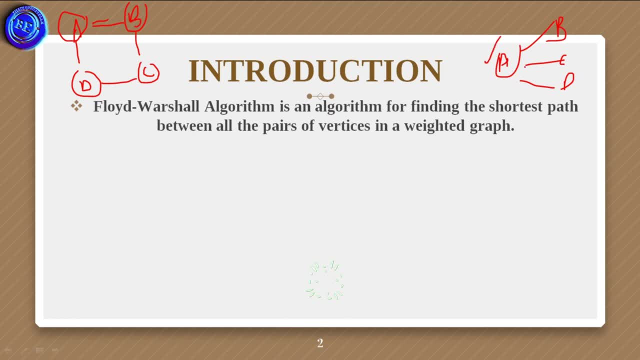 A to C is calculated and A to D is calculated. This is one pair of shortest paths And coming to next vertex B. So from B to A, B to C, B to D. So this is another second pair of shortest path from B to the remaining vertices. 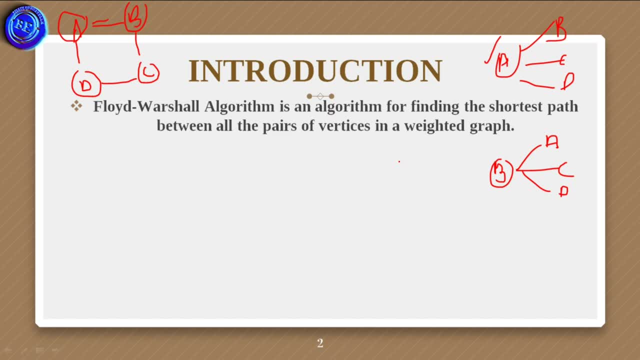 Similarly for C to D. the shortest path for every vertex is calculated in Floyd Verschel Algorithm. This algorithm works for both the directed and undirected weighted graphs. What is a directed graph? It shows a particular direction towards an another vertex, For example, 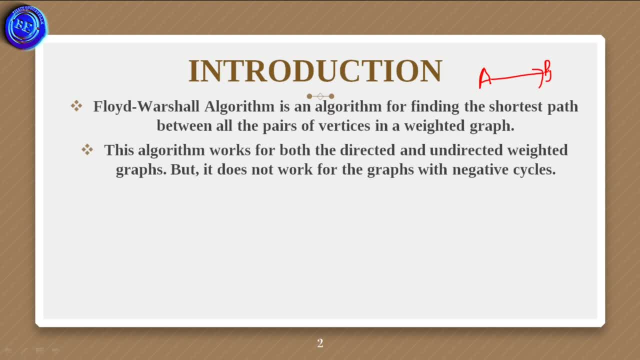 in this direction that means from A to B- the edge value is shown. But in an undirected graph there will be a single line. That means from A to B and B to A. it shows that there are no directions in this type of graphs. But in this graph we have some directions, But it doesn't. 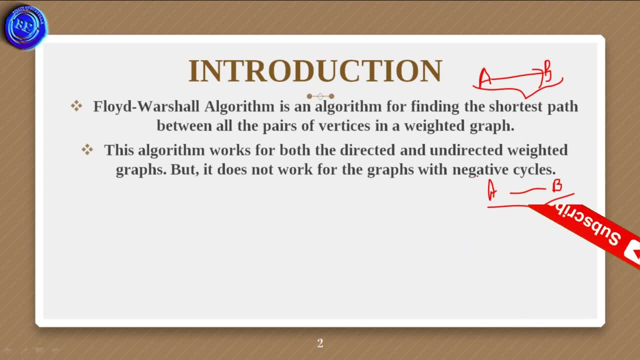 work for the graphs with the negative cycles. What are the negative cycles? When we are going to add the edge values for the shortest path, then the sum of the edge values is equals to negative. Then it is said as a negative cycle When the total edge value of a shortest path is. 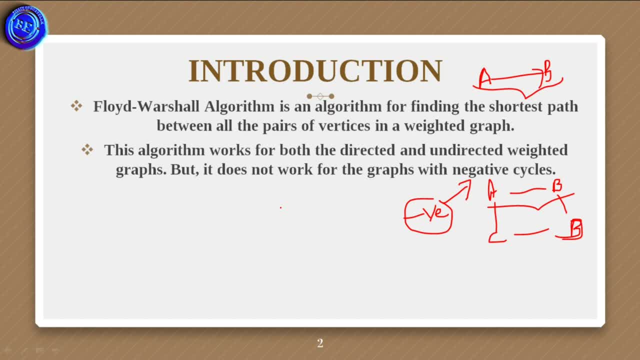 equals to negative, it is termed as a negative cycle. So this Floyd Verschel Algorithm is not work for the graphs with negative cycles. I hope you understood it. This algorithm follows the dynamic programming approach to find the shortest path. What is a dynamic programming approach? 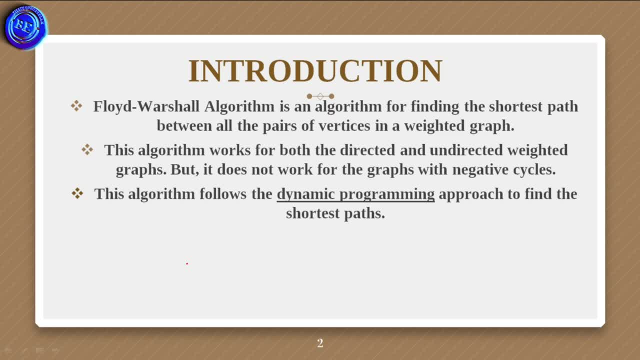 It is like a divide and conquer approach, where we are going to divide the problem into subproblems, But the subproblem solutions are stored in a table, While in divide and conquer we are going to find the solutions repeatedly. Floyd Verschel: Algorithm follows the dynamic. 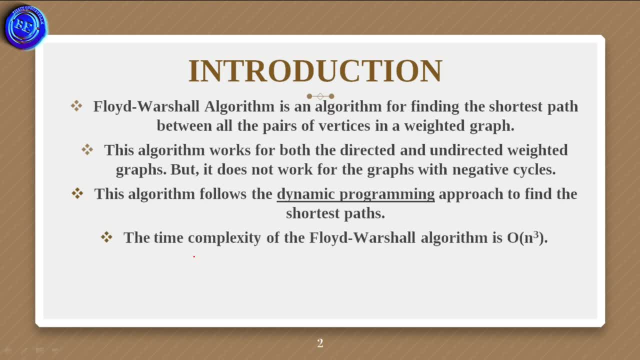 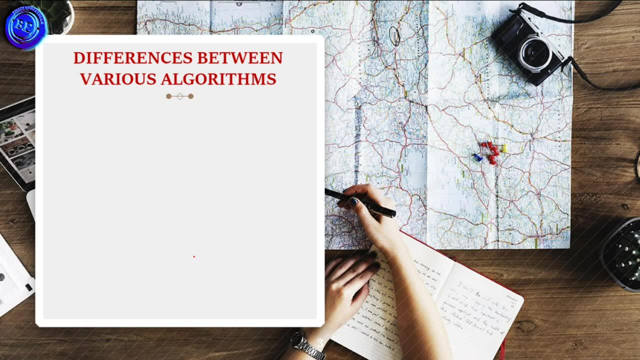 programming approach. The time complexity of Floyd Verschel Algorithm is order of n cube and the space complexity is order of n square. Let us discuss the differences between the various algorithms. As we discussed about the Dijkstra Algorithm, it will find the shortest path from the one node to the remaining nodes. 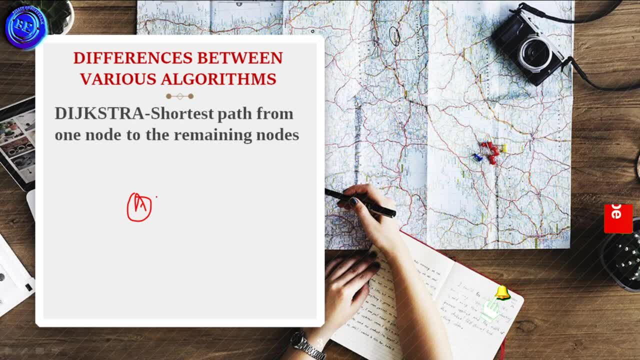 In Dijkstra Algorithm we are going to find the shortest path from one node only. But coming to the Floyd Verschel Algorithm, it will find the shortest path from all pairs of vertices, including the negative edge values. So in a particular graph we have some edge. 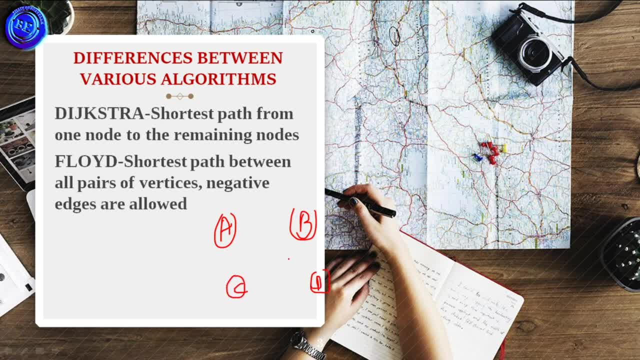 values. So in Floyd Verschel Algorithm we have the negative edge values too. But in Dijkstra we didn't have the negative edge values. But in Floyd Verschel we have the negative edge values and we are going to find the shortest path for all vertices. I hope you understood it. 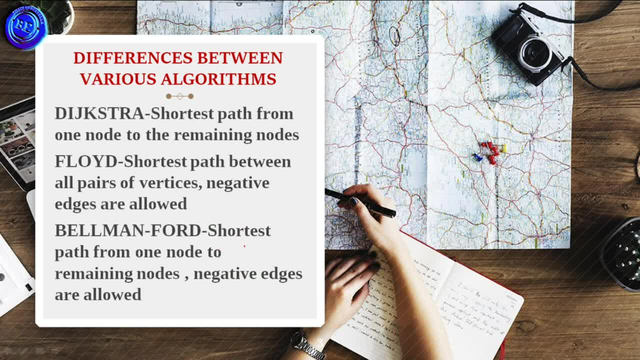 And coming to the Bellman-Ford Algorithm, it will find the shortest path from one node to the remaining nodes, and negative edges are also allowed. So the major difference between the Dijkstra Algorithm and Bellman-Ford is nothing, but the negative edges are added in Bellman-Ford. 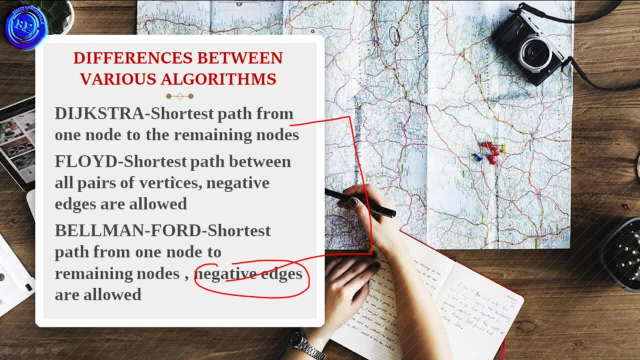 while in Dijkstra Algorithm, negative edges are not present. So in next video session I would like to discuss about Bellman-Ford. Now let us discuss about the Floyd Verschel Algorithm, which consists of negative edges, but it doesn't support the negative cycle. 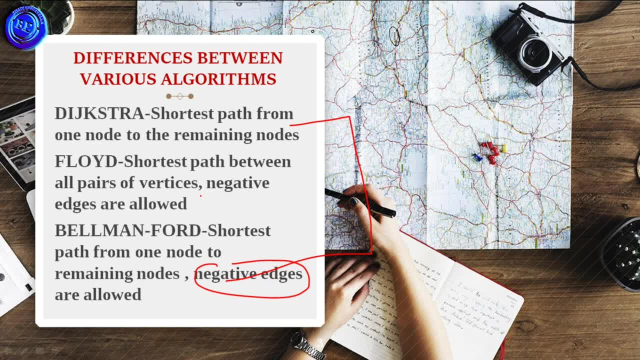 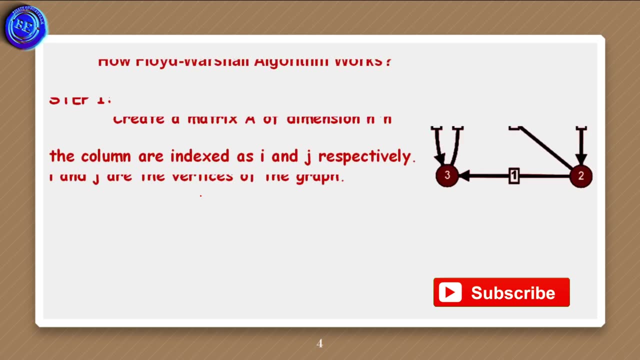 The negative cycle is nothing. but the sum of edge values is equals to negative is termed as a negative cycle. So the Floyd Verschel Algorithm doesn't support the negative cycle, but it supports the negative edge values. I hope you understood it. Coming to, 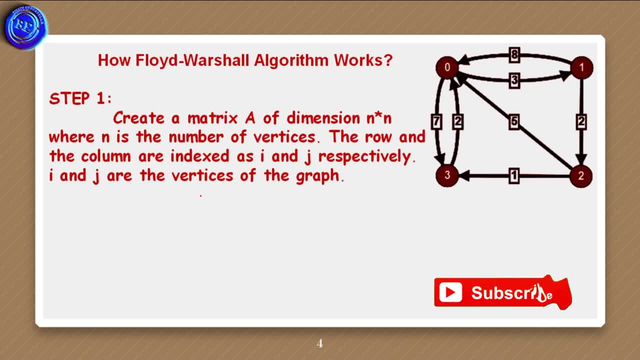 the example. So here I consider a graph. And now let us discuss how this Floyd Verschel Algorithm works. So here I am going to create a matrix named as A, such that its dimension is of size n by n. So here n represents the number of vertices. So here we have four vertices and the row and the. 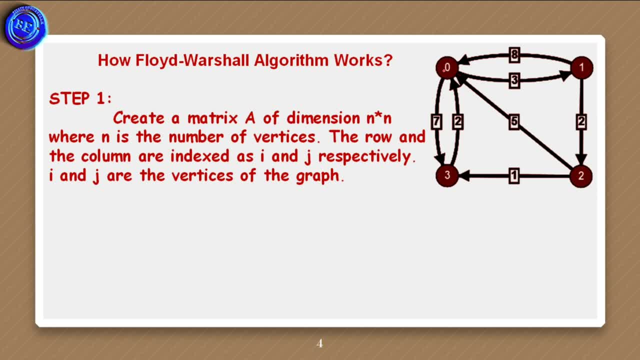 row represents the number of vertices. So here n represents the number of vertices. So here I consider a matrix which consists of the edge values from one vertex to the another vertex, So from zero to zero. we have no edge which is interlinked to it. 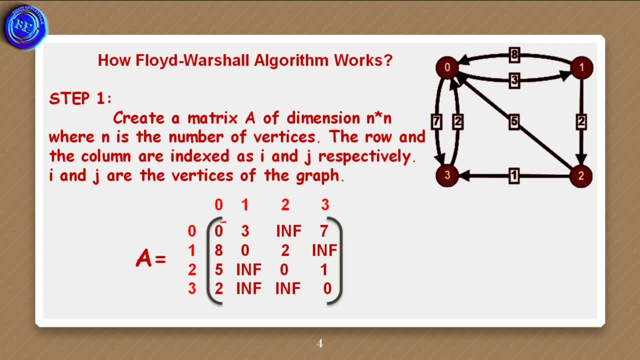 So I represent the diagonal values as zeros. So you can see that the diagonal values are zeros. That means there is no edge value, which is directing towards itself From zero to one. what is the edge value? Its edge value is three, So I represented it as three. 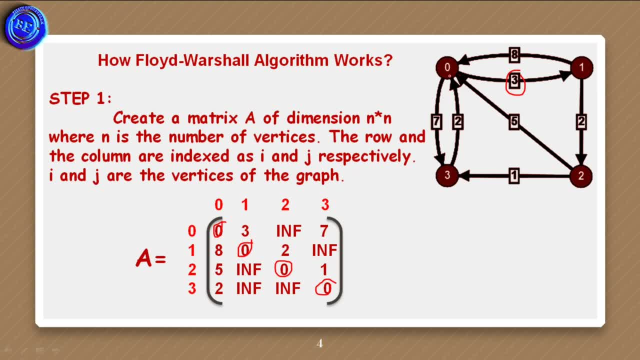 From zero to two. we didn't have any direct edge, So I represented it as inf. inf is nothing but infinity. As the symbol is not possible, I represent it as inf. And from zero to three, the edge value is seven. here you can see that. And from one to zero. from one to zero, the edge. 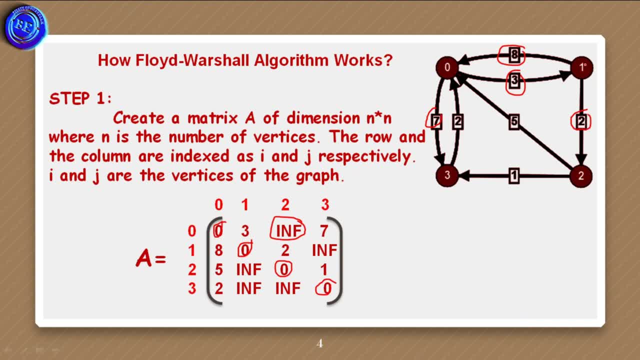 8 and from 1 to 2, the edge value is 2, and from 1 to 3 there is no edge, so I represented it as infinity. and similarly from 2 to 0 the edge value is. so here, from 2 to 0, we have the direct edge. 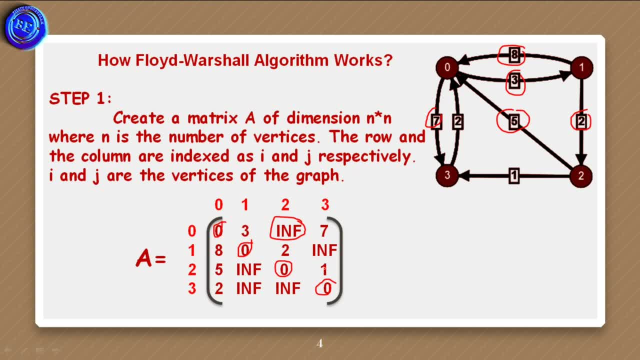 its value is 5, and from 2 to 3 its value is 1. okay, here you can see that. and from 2 to 1 there is no direct edge, so I represented here it as infinity. so similarly you can see the remaining edge values. so in the next step I will say how this Floyd Marshall algorithm works. coming to the 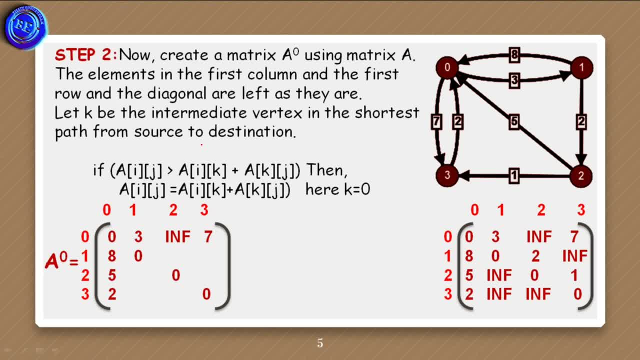 second step. so here in this second step. so here I am going to create a matrix named as a naught by using the matrix a which was derived in the previous slide. so here in this a naught, the first row and the first column and the diagonal elements are same as the previous matrix. that means a. 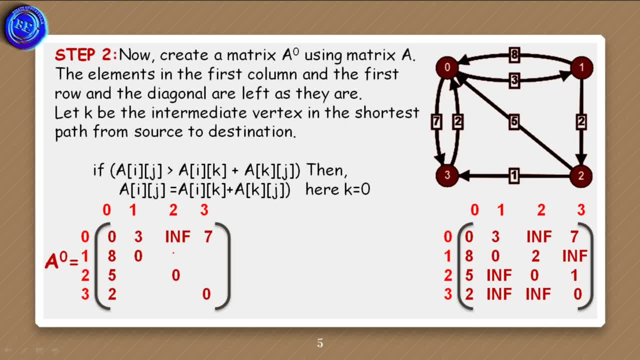 matrix and we are going to calculate the remaining edges by using one intermediate vertex named as K. so initially the K value is 0 as we are taking the a naught, so a naught represents its K value is equals to 0. after, in the next step, we are going to take the K value as 1. in after step we are going to take: 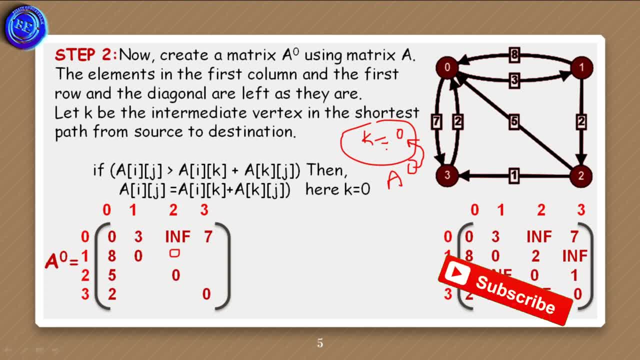 the K value as 2 and in the next step we are going to take the K value as 3. so in every step we are going to increment the K value. so by using this formula we are going to calculate the cost of each vertex. so represents the row, and represents the column, and represents 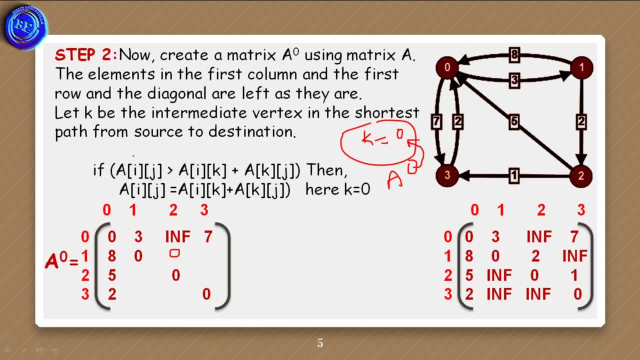 the intermediate vertical. so here for calculating 1st row, 2nd column. so I am representing in as 1 and Jay as 2, and I am going to represent I here as 1 and k value is 0, as i said, and here also k value is 0 and the j value is 2. so 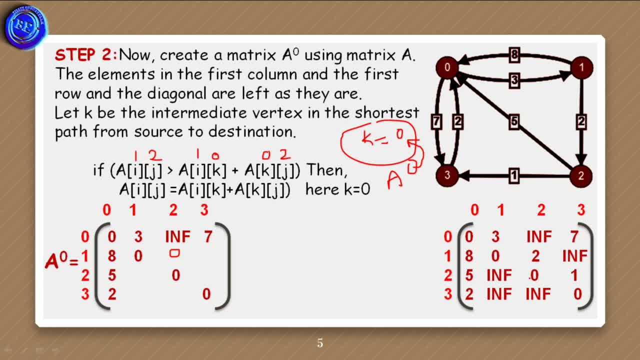 actually, what is the cost of a of 1- 2? so the cost of a of 1- 2 is 2. okay, so please notice it. the cost of edge value between the first vertex to the second vertex is 2, and the cost of first vertex to the 0th vertex is 8 plus and the cost of 0 to second vertex. that means 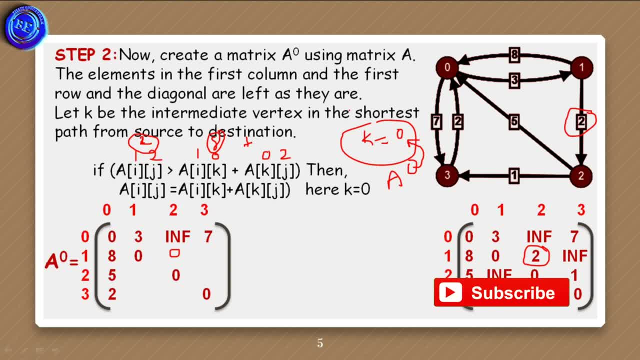 0 to second vertex. its cost is infinity. so infinity plus 8 is nothing but equals to infinity. but here we have one symbol, so actually infinity is greater than 2.. so 2 remains infinity, 15. 17. 18.. 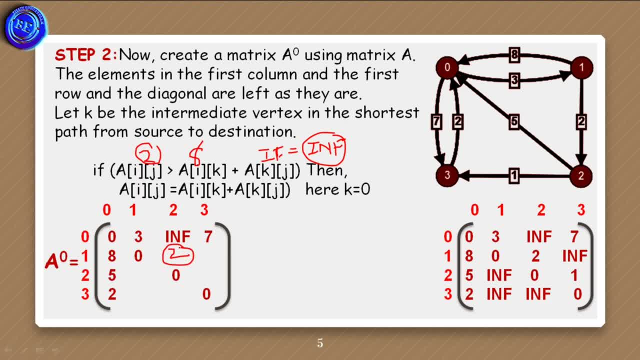 17. 18. 19. 11. its position: okay, so there is no change of this value. and coming to 1- 3: what is the cost of 1- 3? its value is infinite. okay, what is the cost of 1 to 3? its cost. 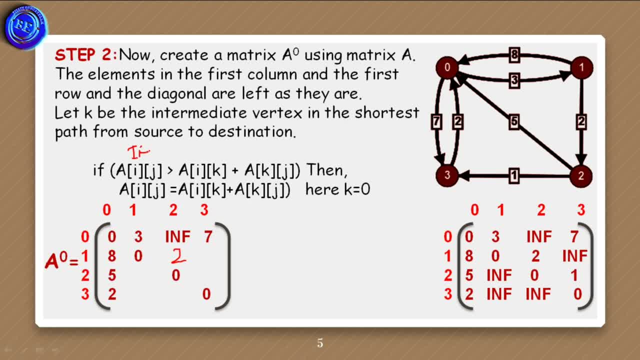 is actually infinite, okay, and the cost of 1 to 0. so here I am representing 1 to 0 and 0 to 3. so here there is a simple tree. when we are taking one to three, it was divided into two halves, that is, 1 to 0 and 0 to 3. this property is known as 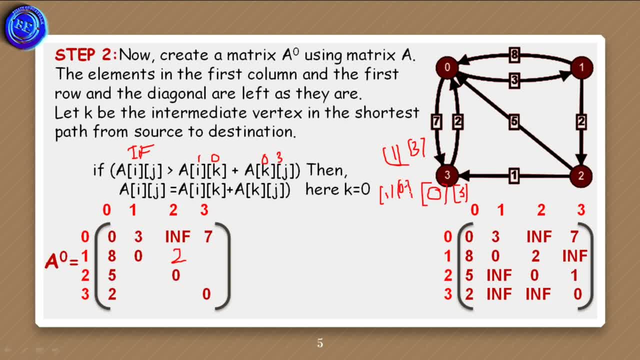 transferred to closure property, which is the basic property of Floyd ships algorithm. so the property which is involved in Floyd Aldersal algorithm is trans to closer property. the cost of 1, 1, 2, 0, 0, 3, 0 is 8 and the cost of 0 to 3 is 7. so actually the infinity is greater than the cost of. 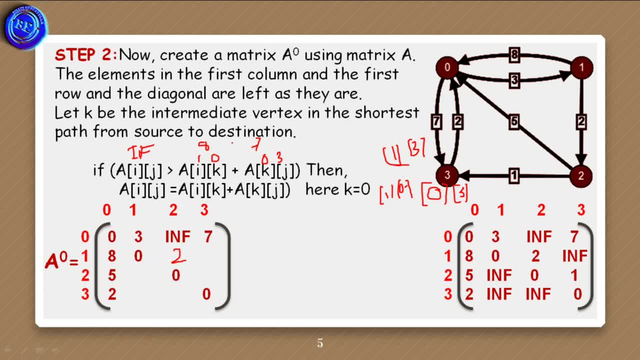 1 to 0 and 0 to 3. when they are added, its value is equals to 15. so 15 is updated here. i hope you understood it. next, similarly 2 to 1. so 2 to 1 means first it is going to find the cost from 2. 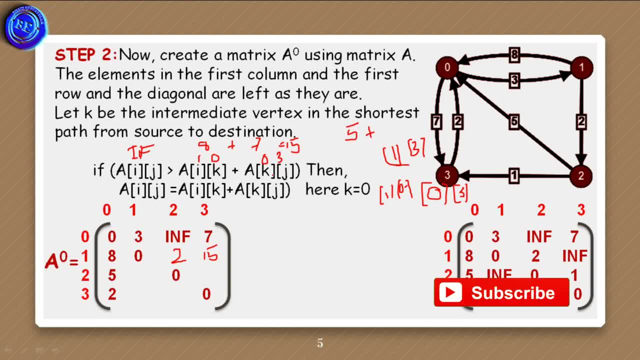 to 0, its cost is 5, and from 0 to 1 its cost is 3. so 5 plus 3 is 8. so here 8 is updated. i hope you understood it. and similarly for 2 to 3. first it is going to find the cost from 2 to 0, after that. 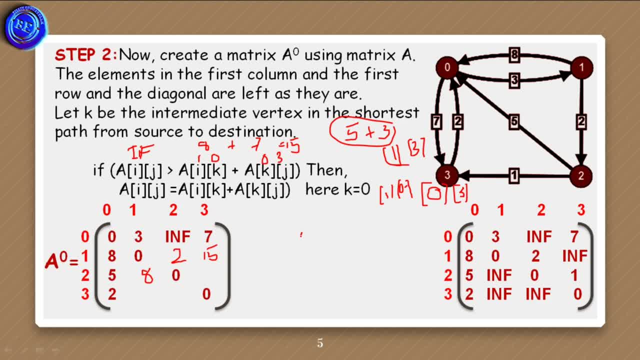 0 to 3. what is the cost of 2 to 0? its cost is 5. and from 0 to 3, what is its cost? its cost is 7. actually, the cost of second or third column is 1. so 1 to 1 is 8, and from 0 to 3 it is 7, and from 0 to 3 it is 7 and from 0 to 3 it is 8 and from. 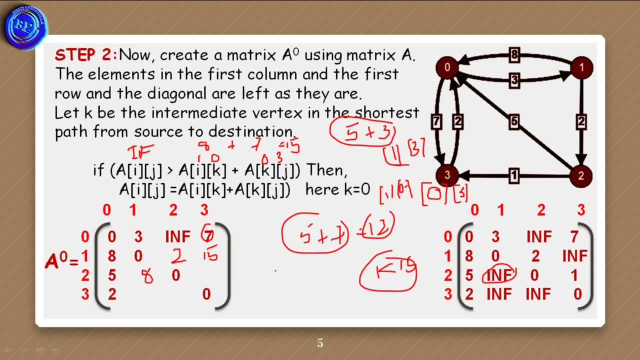 1 is less than 15, so 1 remains in its position. next 3 to 1. so first it will calculate the cost of 3 to 0. its cost is 2, and from 0 to 1 it calculates its value. its value is 3, so 2 plus 3. 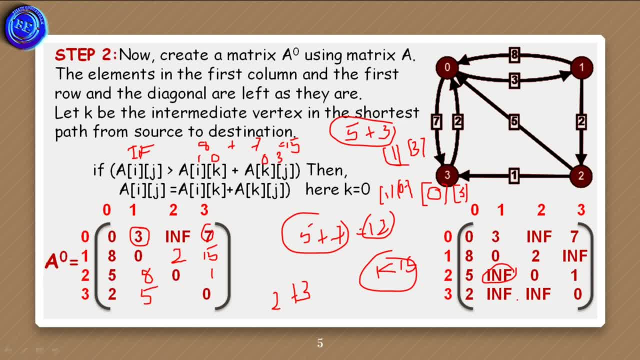 its value is 5. it is updated here and next coming to 3 to 2. so from 3 to 0 its value is 2 plus and from 0 to 2 its value is infinite. the cost of third row, second column, is infinite. 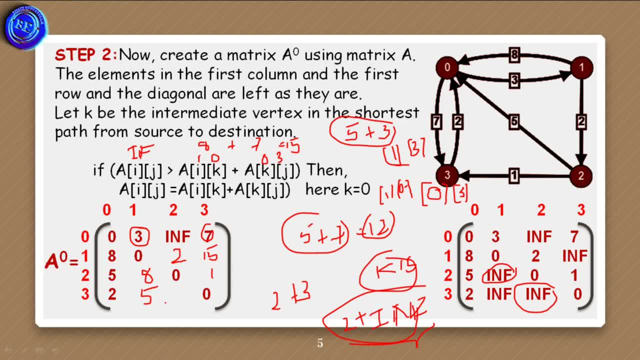 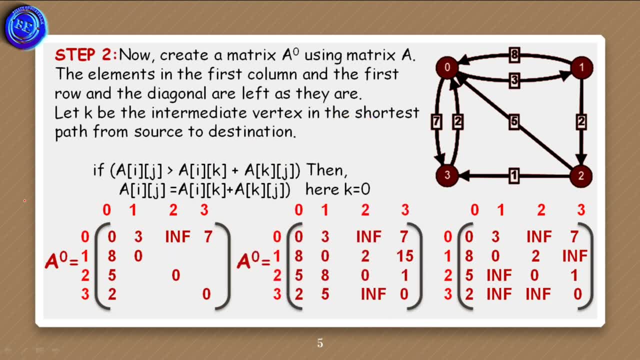 and the calculated value is also infinite. so here we are going to represent the infinite value as it is. so here i am going to represent the matrix. so the updated values are first row and third column. so here 15 is updated in place of infinite, because the cost is minimum value. 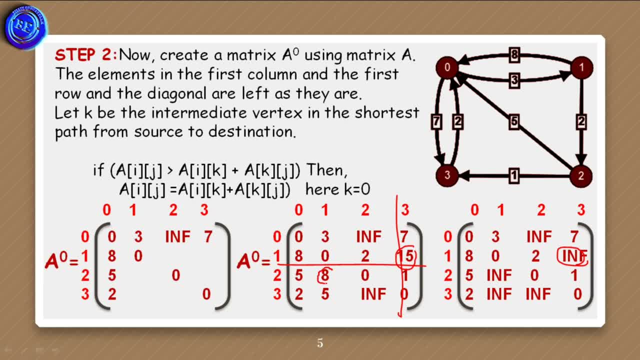 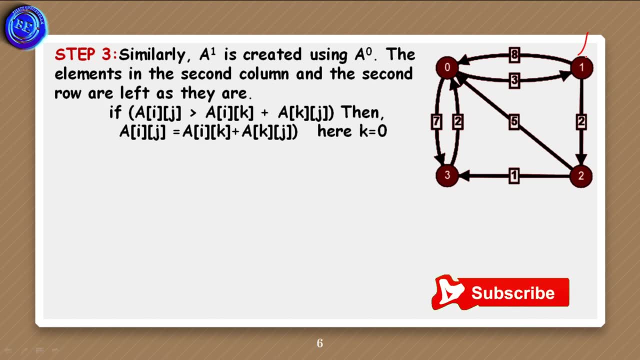 when compared to infinite, and here 8 is updated in place of infinite, and here 5 is also updated. and coming to the next step, here we are going to take the first vertex. that means this vertex is considered as an intermediate. okay, so k value is equals to 1 and i and j values represents the. 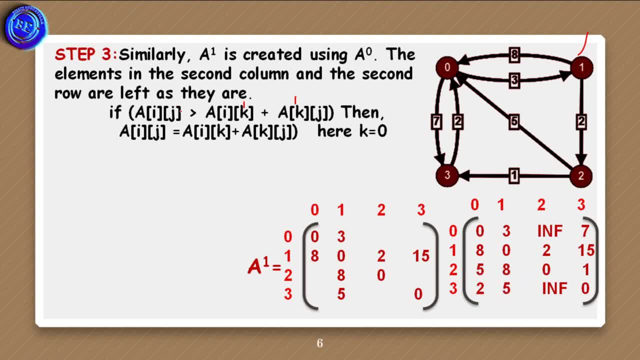 rows and the columns. so here we have the matrix. so this is our previous column and we are going to take the next column and we are going to take the next column matrix. that was done in step 2, so by using the previous matrix only we are going to calculate. 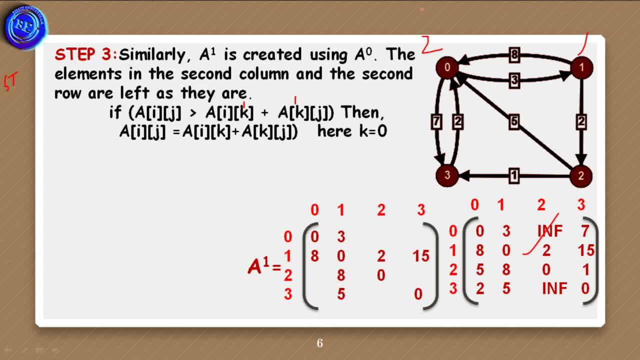 the next matrix. so for step 2 we have to take the matrix of first step. for calculating the third step, we are taking the matrix of second step. so for calculating the values we are keeping the first row and the first column and the diagonal elements as it is, and here we are going to update the values. 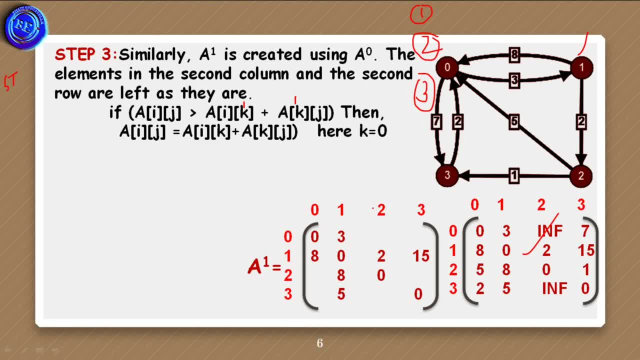 first we are going to calculate the value from 0 to so, 0 to so. what is the cost of 0 to- actually it is infinite- and the cost of the intermediate. that means 0 to 1 plus 1 to 2. okay, what is the cost of? 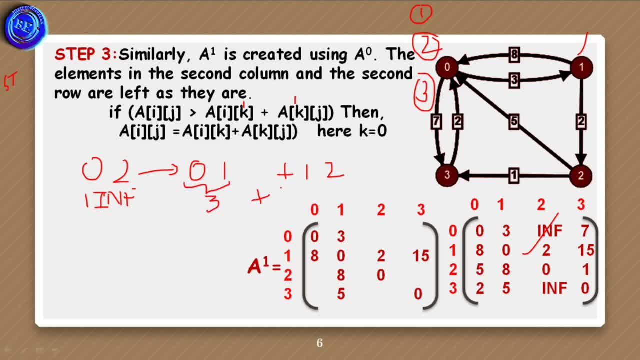 0 to 1. its value is 3 plus. what is the cost of 1 to 2? that means 1 to 2. what is its cost? 2? so 5 is updated here. I hope you understood it. and coming to the next one, 0 to 3. okay, 0, 3, so the 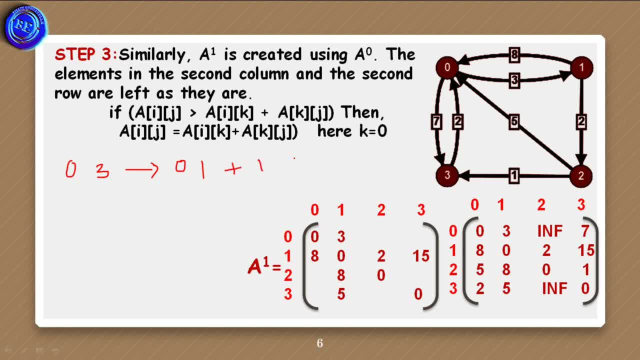 intermediate vertex is 0 to 1 plus 1 to 3. what is the cost of 0 to 3? its cost is 7. what is the cost from 0 to 1? its cost is 3 plus. what is the cost from 1 to 3? its cost is 15. so this value is: 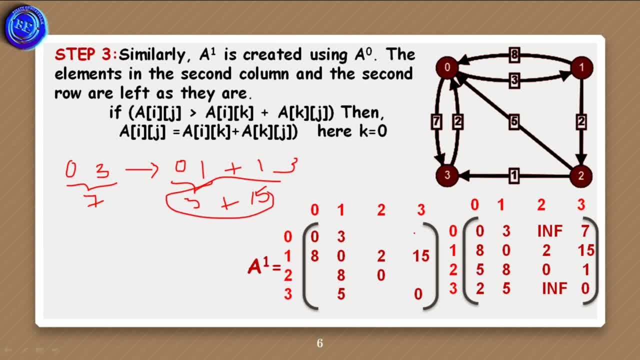 greater than 7, so 7 remains in its position. okay, second row, 0th column, so 2: 0. the intermediate vertex is 1 to 1 plus 1 to 0, so what is the cost of this? its cost is 5, so what is the cost of 2 to? 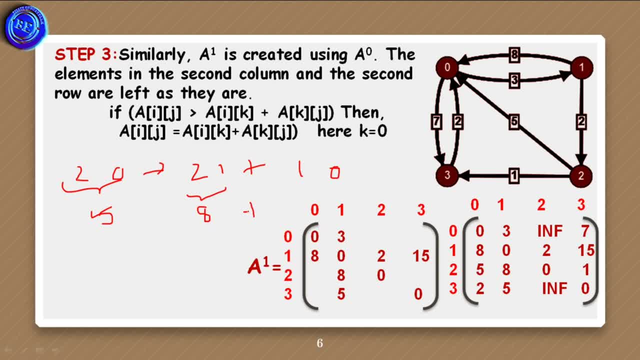 1, its cost is 1 plus. what is the cost of 1 of 0? its cost is 8, so this value is greater than 5, so 5 remains as it is. and next coming to 2 to 3, so two to 3, so the intermediate vertex is 1, so the intermediate vertex is 1 and 1, 2, 3, what is the? 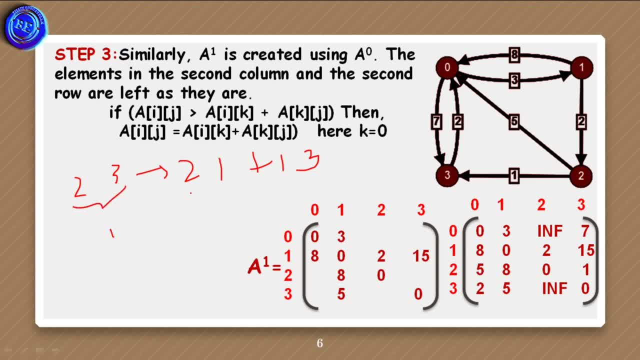 cost of 2 to 3. its cost is 1, and 2 to 1, its cost is 8, and 1 2 3, its cost is 15. so 1 ≤ 1 ≤ 23, so 1 remains in its position, next coming to 3 to zero. so 3 to zero is. 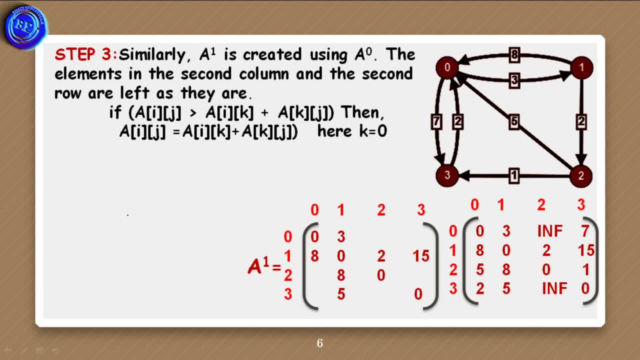 also remains same and coming to 3 to 2. so third row, second column, equals to 3 to 1 and 1 to 2. what is the cost of 3 to 1? its cost is 5 plus what is the cost of 1 to 2? its cost is 2, so 5 plus 2. 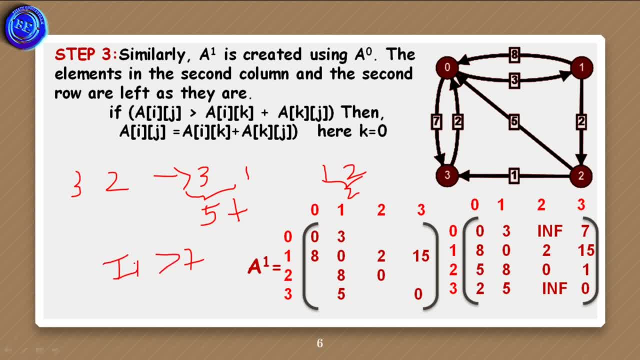 7. 7 is less than infinite, so 7 is updated here. i hope you understood it. so the matrix in the third step is represented here. so here the updated value is 7 and the second updated value is 5. so in place of infinite, we are going to update the values and coming to the next step. 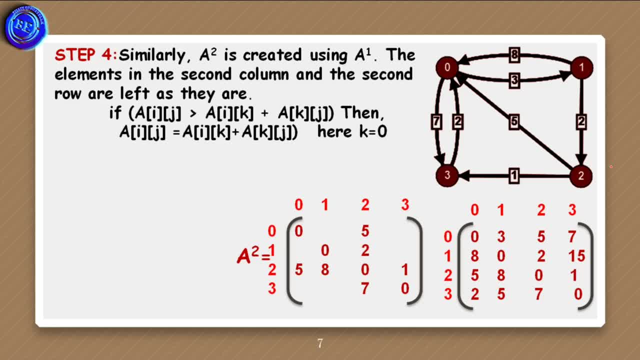 we are going to take the second vertex similarly in the previous steps, as i discussed. so 2 is taken as the intermediate between the two vertices. so the second row and the second column. so here second row means this row. so i represented 2 as the second row and 3 as the third row and 1 as the first row. 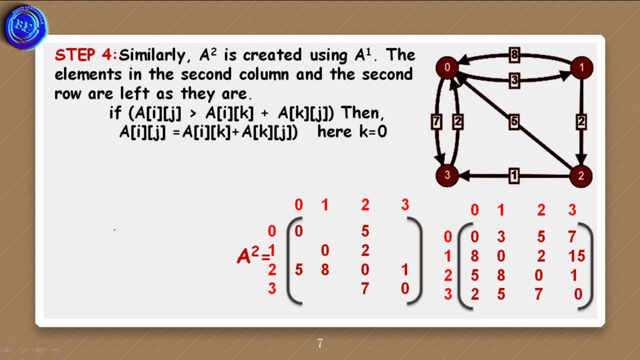 and 0 as the zeroth row. okay, the matrix for the fourth step is as follows: here you may notice that 0 as the zeroth row and 0 as the zeroth row, and 0 as the zeroth row and 0 as the zeroth row. 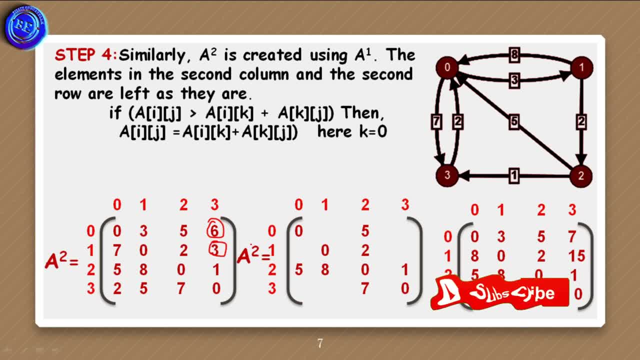 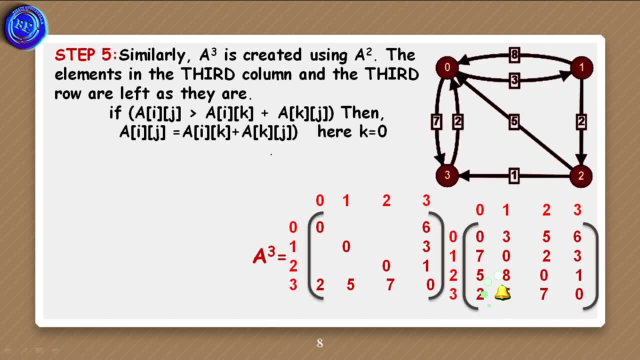 this and this values are changed and the remaining values are as this. coming to the fifth step in this step, 3 acts as the intermediate between the two nodes. so here, third, vertex acts as the intermediate. so after calculating the values here i am representing directly. so at 2, 0, its value is: 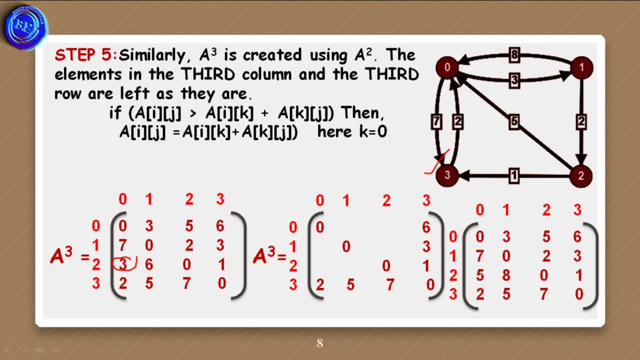 changed to 3, actually the value is changed to 3, so here the value is changed to 3, so here the value is 5, but it was changed to 3, and the 2- 1 is also changed. actually its value is 8 and it. 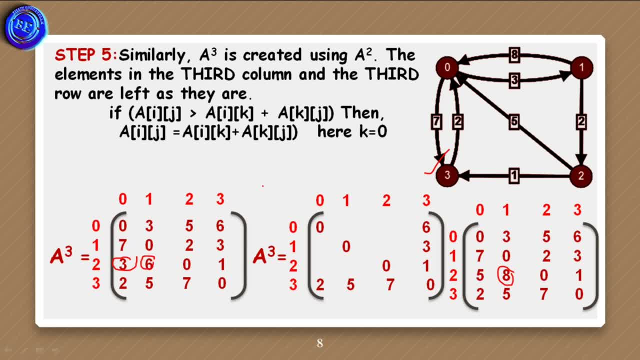 is updated to 6. so by using the full virtual algorithm and the formula, we calculated the shortest paths for all the vertices. i hope you understood it. and here you may notice that from 0 to 0 there is no edge, so it is represented as 0. from 0 to 1: the shortest path is 3. from 0 to 2: the 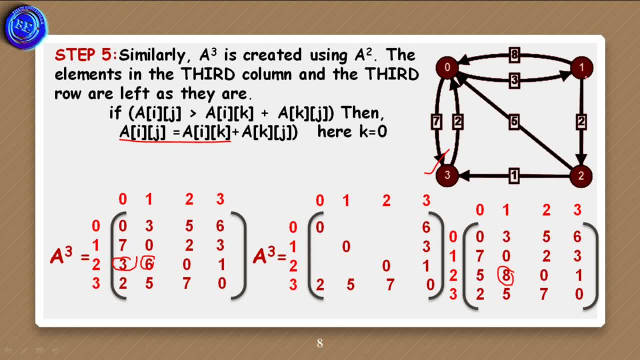 shortest path is 5. that means from 0 to 2, means first it's travel from 0 to 1 and then travels from 1 to 2, and coming to 0 to 3, it will travels from 1, 0 to 1 and 1 to 2 and 2 to 3. so in this way, 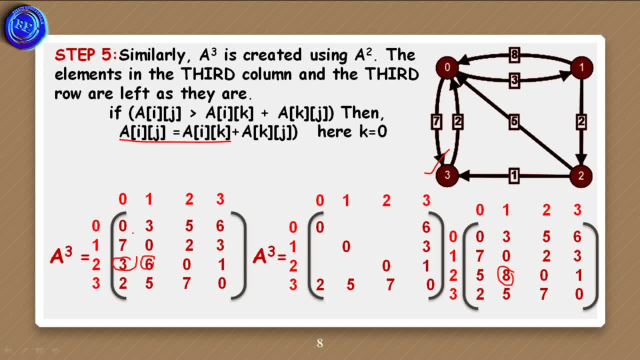 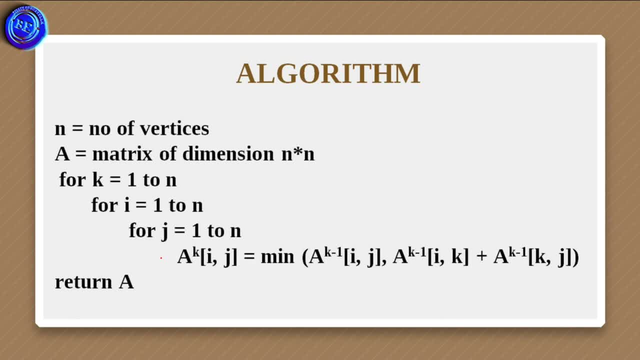 the shortest paths is calculated for every pair of vertices. now let us discuss the algorithm for floyd version. so here we have n vertices and a matrix of dimension n by n. so in that matrix we are going to take the k value and i value and j value. k represents the intermediate between the 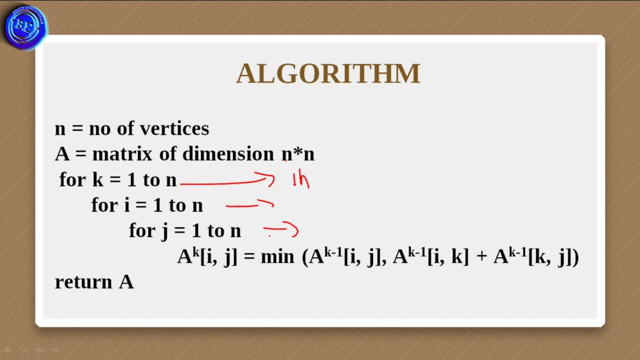 vertices and i represents the row and j represents the column. so here we have the formula. so by calculating the minimum, we are going to update the value in that particular matrix and return the value in the particular matrix, and return the value in the particular matrix and return. 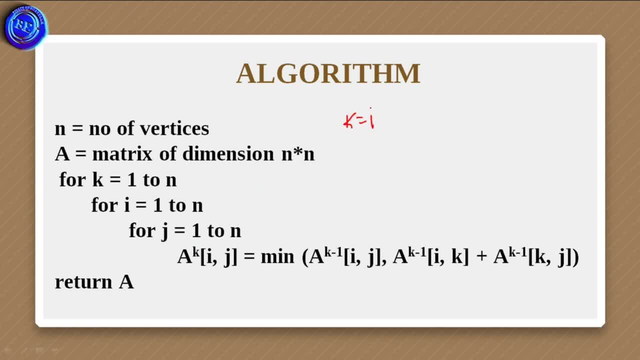 that value. so if i consider the k value is equals to 1, then i comma, j values are also 1 and 1. so first, initially, the i value remains constant and the j value is incremented. that means 1, 2, 3 and 4. okay, as we take four vertices. after calculating the j values again, it comes back to i and i value.